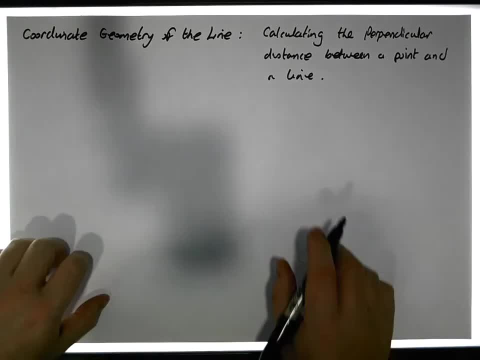 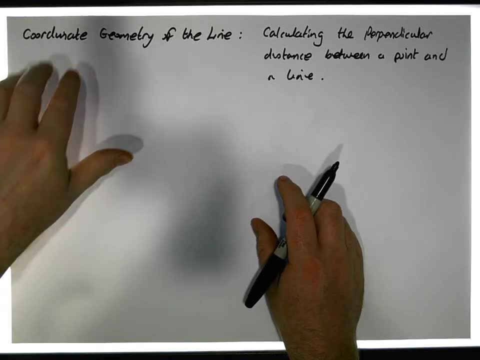 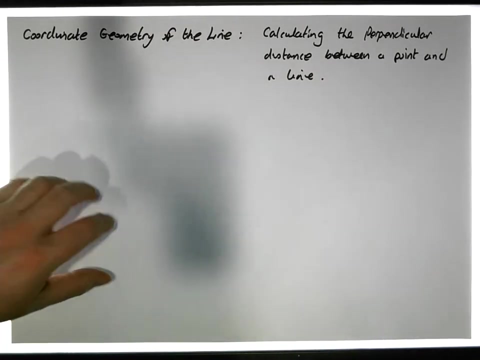 Hi guys, this is Jonathan Lambert with the Mathematics Development and Support Service at the National College of Ireland, and this short video- another video in our series of videos dealing with coordinate geometry of the line- this time is going to deal with calculating the perpendicular distance between a point and a line. So this particular example, let's say for 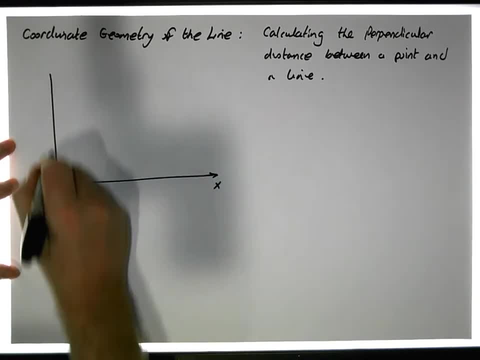 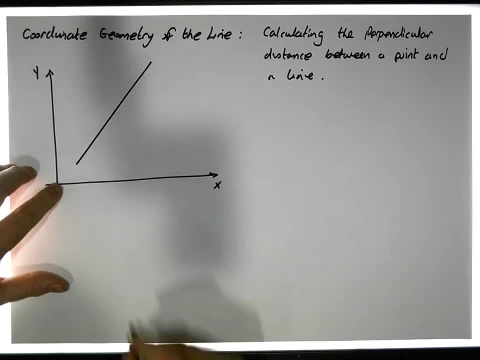 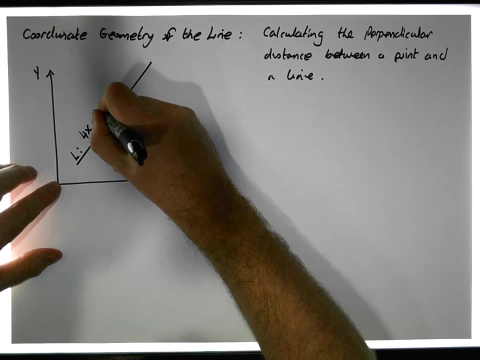 argument's sake, that we have an x-axis, and let's say we have a y-axis. and let's say that we have a line that has positive slope. here's a line with positive slope. let's say L and let's say, for argument's sake, that L has the form it's. let's say 4x minus 3y. let's say plus 4, plus 4. 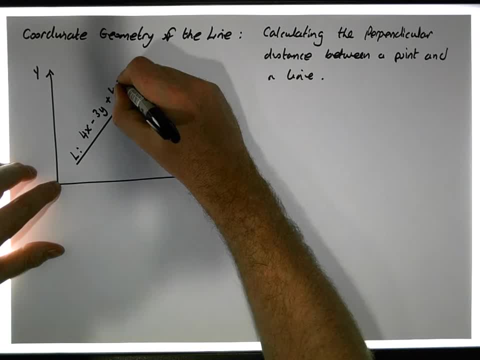 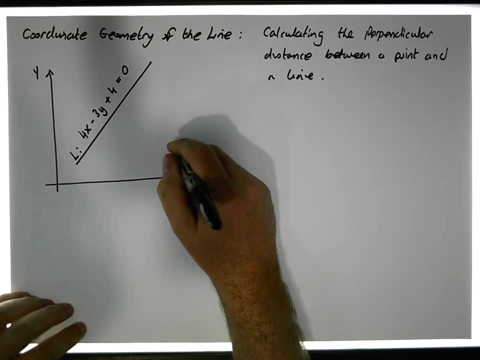 is equal to 0, let's say is equal to 0, so there's a positive sloped line here and let's say we have a point. the point, let's say, is: let's say the point is over here somewhere. let's say the point. 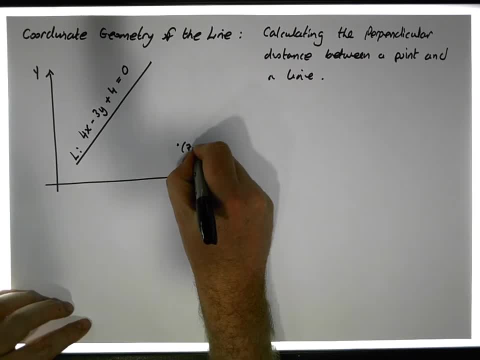 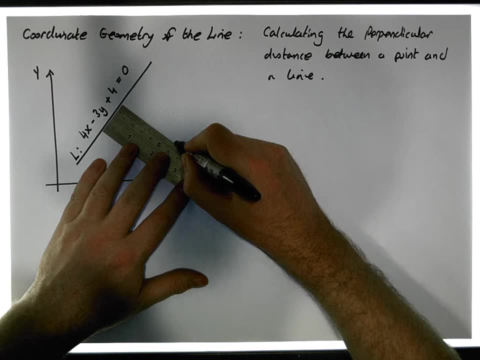 is 7,, 7,, 2, let's say for argument's sake, okay, and what we'd like to do is we'd like to calculate the perpendicular distance between the point and the line. so we'd like to calculate how far this. 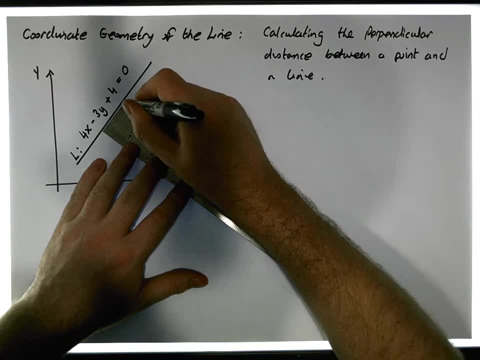 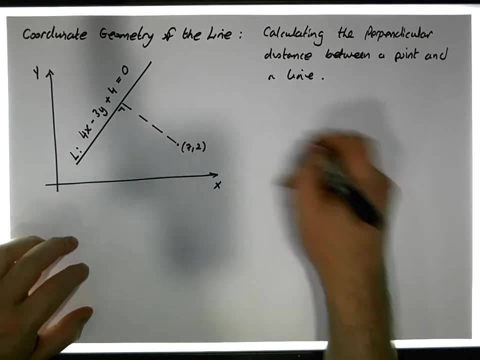 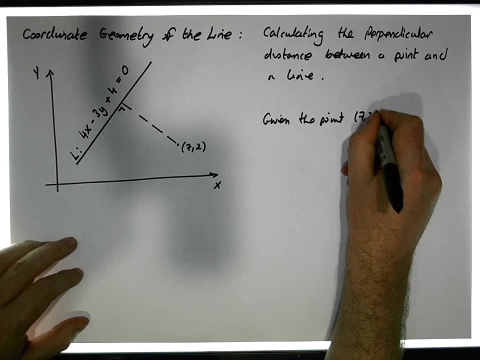 particular point is away from this particular line here. okay, and in particular, the perpendicular distance. okay, so we have a line L and we have a point 7, 2, so maybe this would be something like this: given given the point, the point 7, 2, okay, and the line L and we have a point 7, 2,. 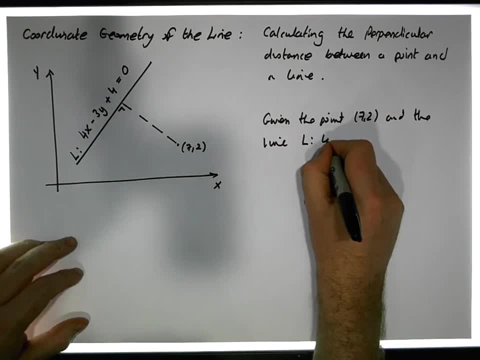 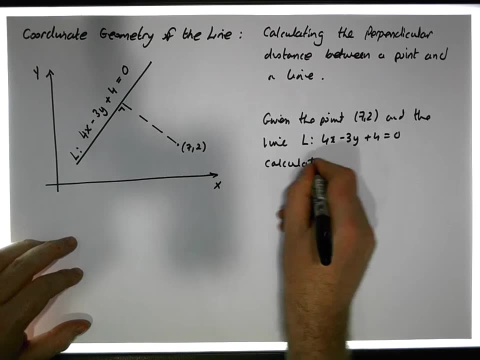 7, 2, length 9,. this is a line times 5,, 5,, 6,. ok, and this could be the point 7, 2,, 6,, 8, where the point 7, 2, 7, is the one that plays out via a line that's not fixed to it. ok, so we'reis. 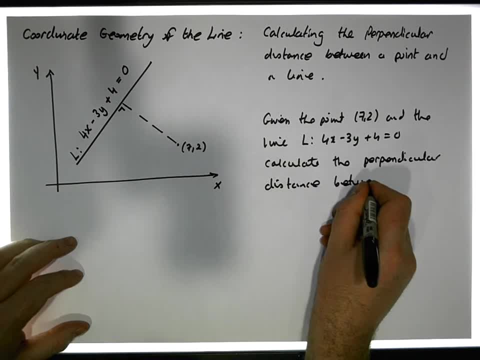 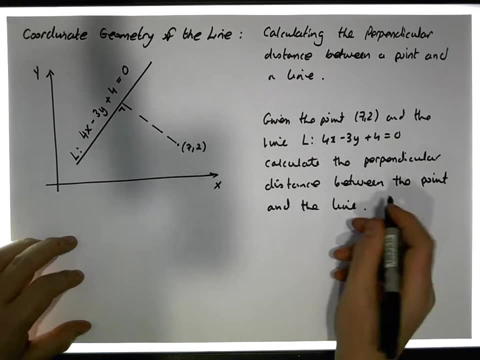 till we punctuate this hetero one of these steps, when we're back to the regular form, and we'rein fact that the point is so this line here. we'rein fact that the point page is the other integral I times 4.. 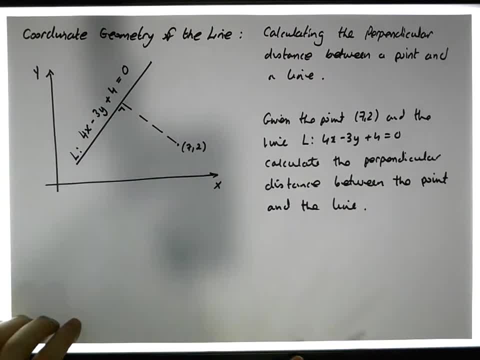 So that's how we need it to be- Of which we need to find out. where is it placed on line 1. dollars per minute. okay, so in fact, this is the time at which the point paid business plot the point. okay. so when you're going to answer these questions, it's nice to actually 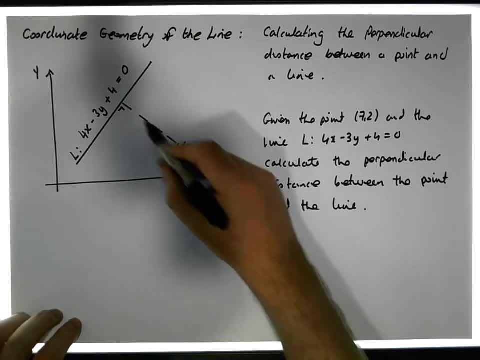 visualize what they look like. okay. so here's the line l and here's the here's. let's say the point 7, 2. so why don't you go off and why don't you plot the line and why don't you put the point relative to the line and show what you mean by the perpendicular distance? okay, and then let's. 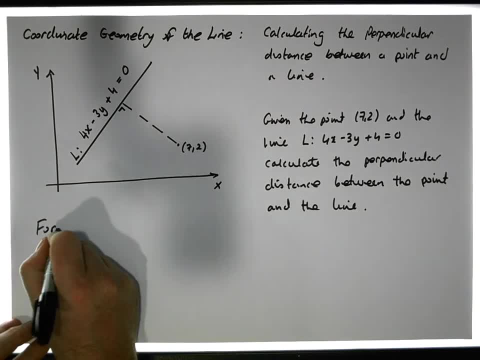 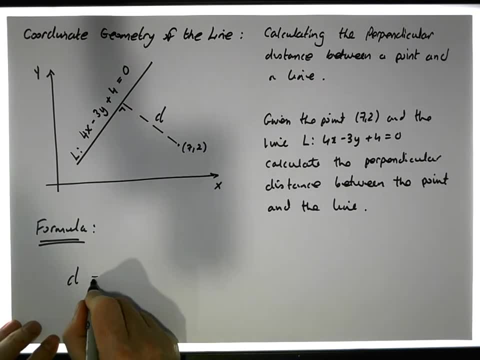 use the formula. the formula says: okay, the formula, okay, okay, which is really straightforward. the formula says that the distance, okay, that this distance here, d, okay- is simply equal to the absolute value of ax, 1 plus by 1 plus c, divided by the square root of a squared plus b squared. 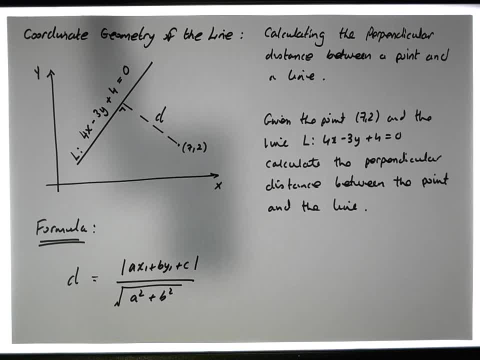 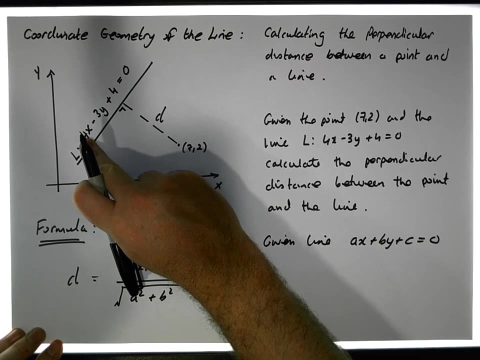 that's the square root of this here. okay, so all we need to know is the coefficients ab and c. okay, the coefficients of the line. so, given the line, the line ax plus by plus c is equal to zero. they're the coefficients abc. we have a 4 minus 3, 4. okay so. 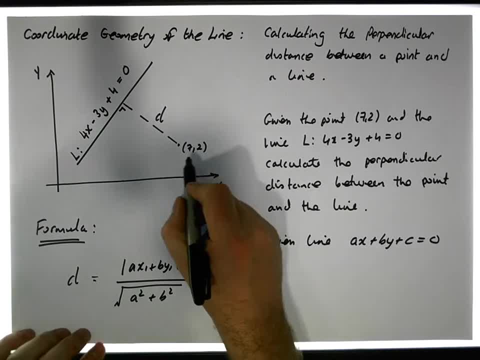 all we need is the coefficients uh, az and c. okay, so all we need is the coefficients b and c. okay, so all we need is the coefficients a, a, a, b, c, dude, thank you. thank you very much, commercially y believingiant people. okay, your b and c, and we need a point x1 y1. okay, here's our point x1 y1. uh, here's our a, here's our b, here's. 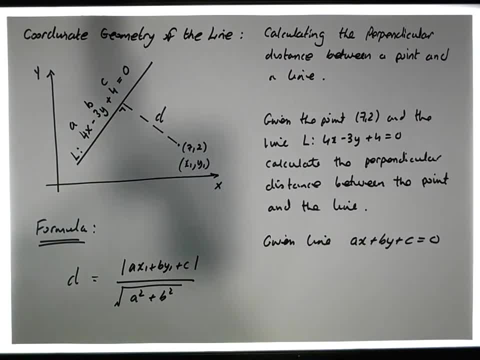 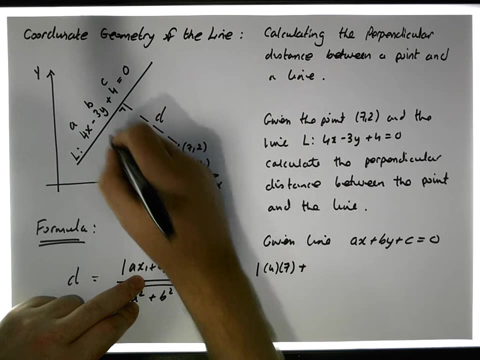 our c, so we can actually just substitute them into this formula and we have, and we have our solution. okay, so this becomes, this becomes the absolute value uh of a, which is four times x1. x1 is seven, so four times seven uh plus b. well, b in this case is minus three, so it's minus three. 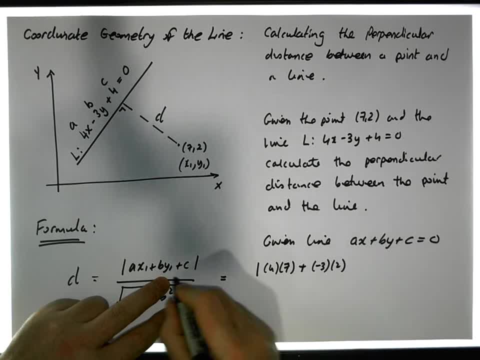 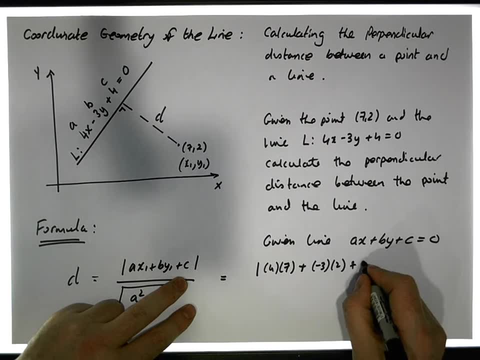 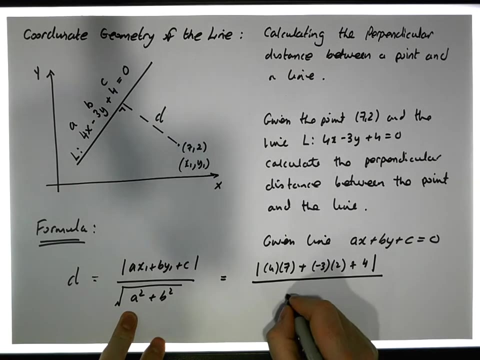 times y1. y1 is two, okay, and it's going to be plus our c, the constant term in our equation of our line, which is actually a plus four here. so it's going to be plus plus four and it's the absolute value of that divided by the a squared. well, the coefficient of the x term here is four, so it's. 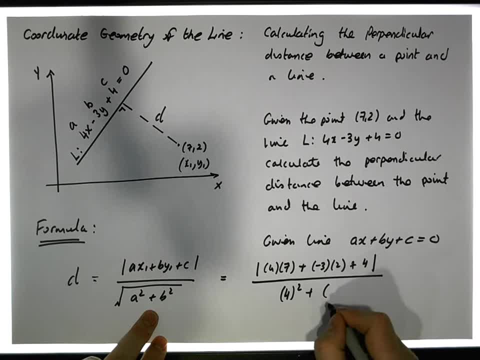 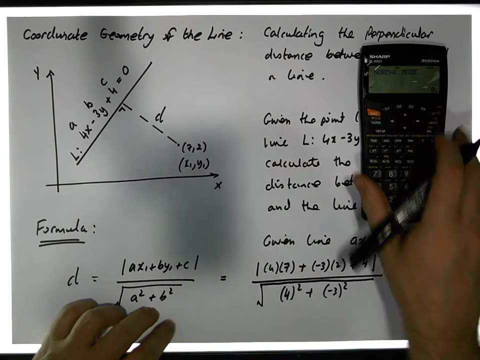 got to be, it's got to be four squared, uh, plus plus the b value. the b value is minus three. so it's minus three to be squared and it's the square root of that. so it's the square root of that term there, right, which gives us a value. so let's just grab our calculator, so the calculator here will tell us that. 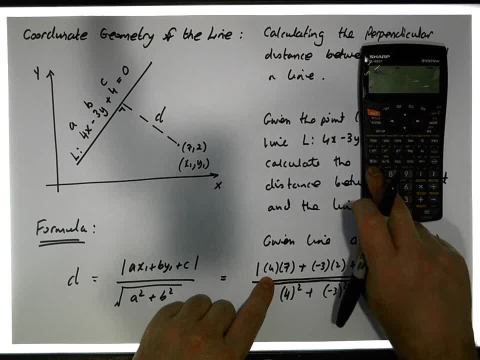 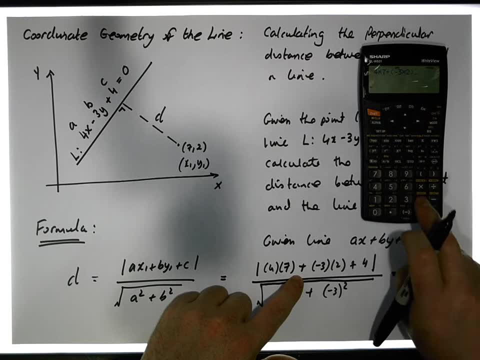 well, let's see what we have. so we have it's 4 times 7,. 4 times 7, it's going to be plus it's a negative 3, so it's a negative 3 times 2, okay, plus 4, it's going to give.